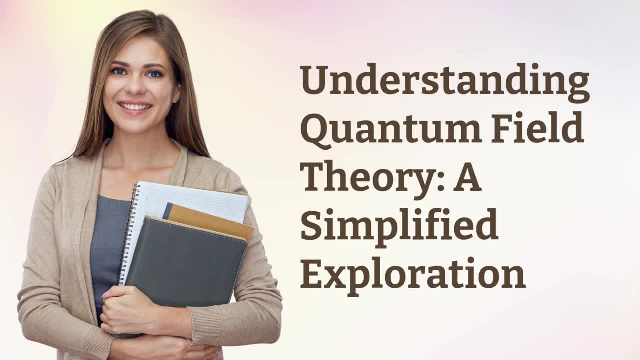 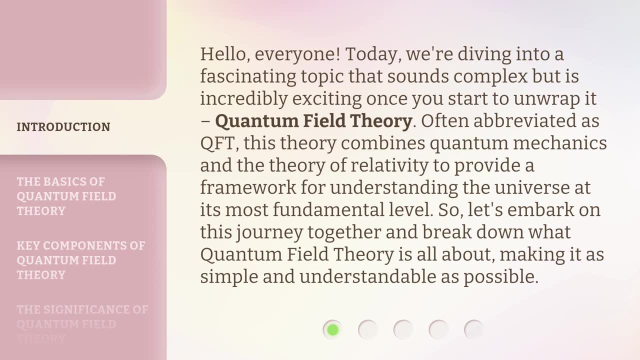 Understanding Quantum Field Theory – A Simplified Exploration. Hello everyone, Today we're diving into a fascinating topic that sounds complex but is incredibly exciting once you start to unwrap it – quantum field theory, Often abbreviated as QFT. this theory combines quantum mechanics and the theory of relativity to provide a framework for 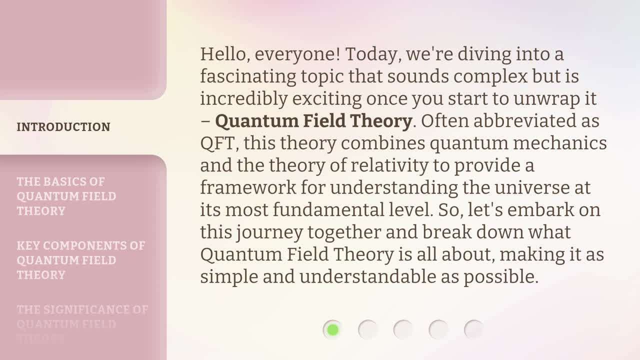 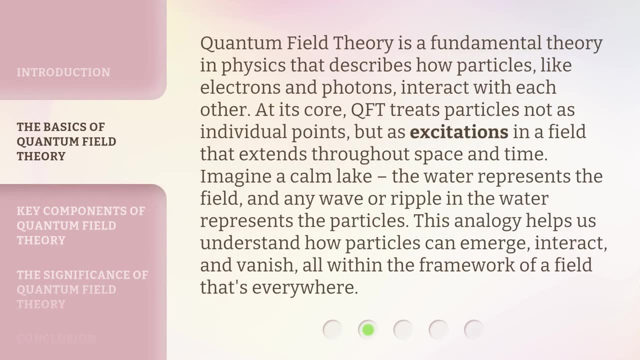 understanding the universe at its most fundamental level. So let's embark on this journey together and break down what quantum field theory is all about, making it as simple and understandable as possible. Quantum field theory is a fundamental theory in physics that describes how particles 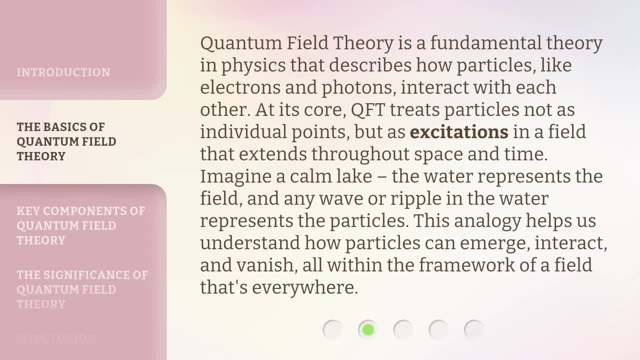 like electrons and photons, interact with each other. At its core, QFT treats particles not as individual particles, but as particles that interact with each other. QFT treats particles not as individual points, but as excitations in a field that extends throughout. 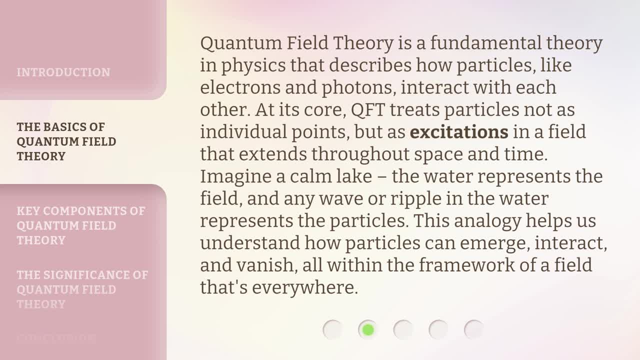 space and time. Imagine a calm lake. The water represents the field and any wave or ripple in the water represents the particles. This analogy helps us understand how particles can emerge, interact and vanish, all within the framework of a field that's everywhere. 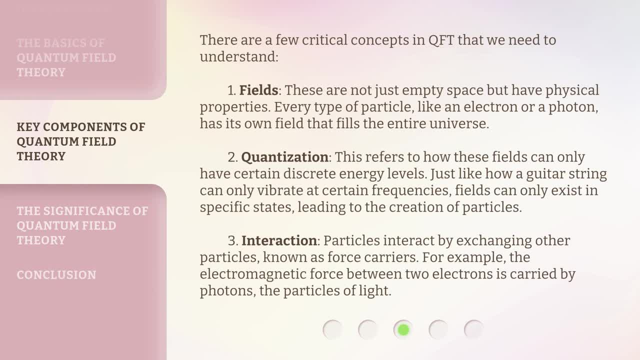 There are a few critical concepts in QFT, and they are the following: 1. Fields: These are not just empty space, but have physical properties. Every type of particle, like an electron or a photon, has its own field that fills the entire. 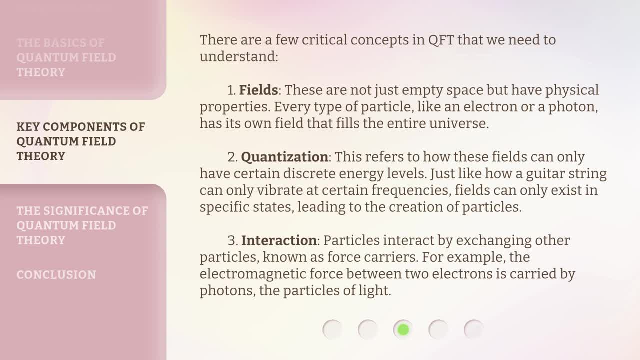 universe. 2. Quantization: This refers to how these fields can only have certain discrete energy levels. Just like how a guitar string can only vibrate at certain frequencies. fields can only exist in certain frequencies. 2. Quantization: This refers to how a guitar string can only vibrate at 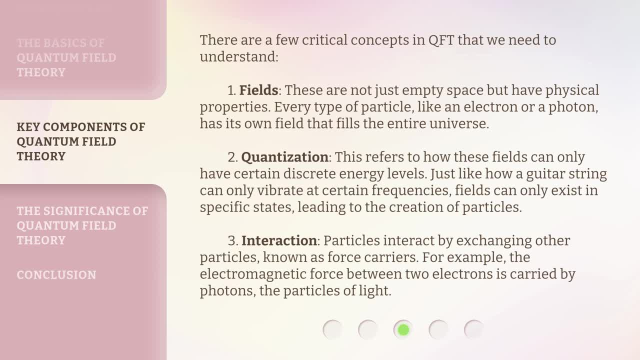 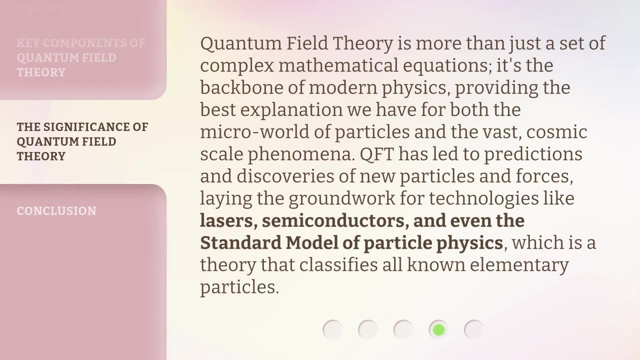 specific states, leading to the creation of particles. 3. Interaction: Particles interact by exchanging other particles known as force carriers. For example, the electromagnetic force between two electrons is carried by photons, the particles of light. Quantum field theory is more than just a set of complex mathematical equations. It's the backbone of modern